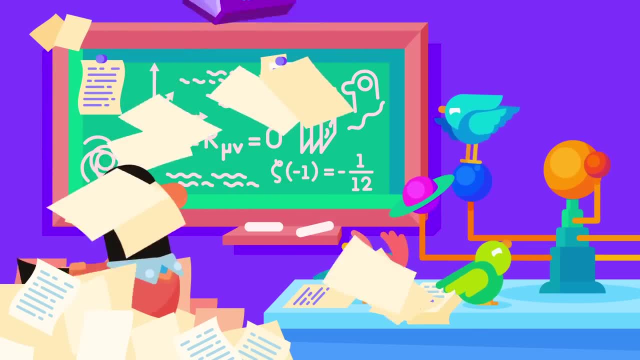 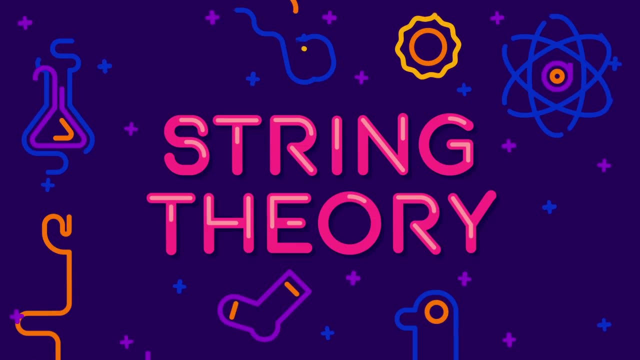 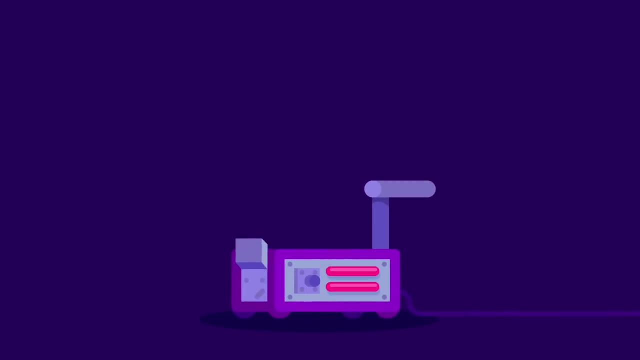 Some of them so much so that it's really hard to know what they're actually about. Like string theory, A famous, controversial and often misunderstood story about the nature of everything. Why did we come up with it, and is it correct or just an idea we should chuck out? 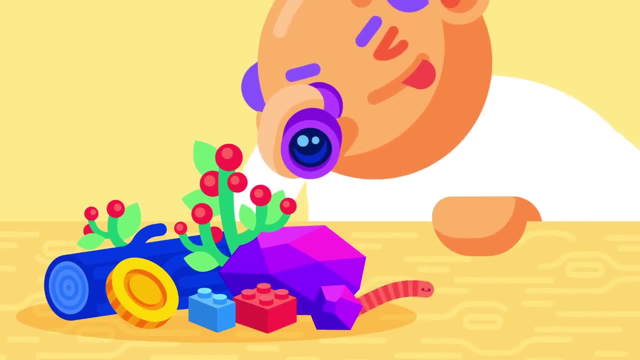 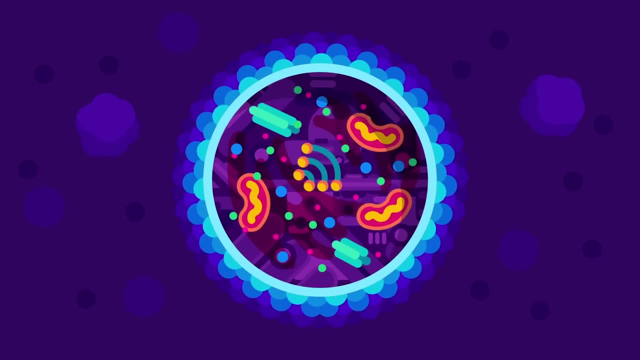 To understand the true nature of reality. we looked at things up close and were amazed: Wondrous landscapes in the dust, Zoos of bizarre creatures, Complex protein robots, All of them made from structures of molecules made up of countless, even smaller things. 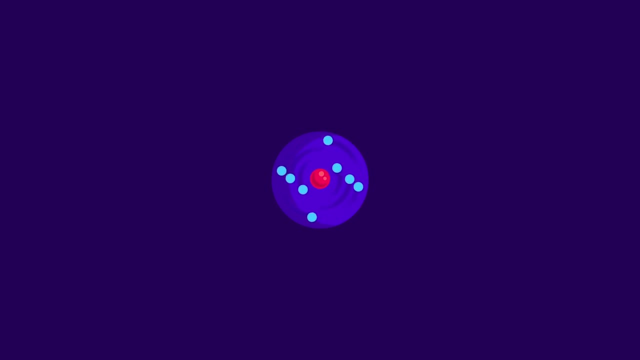 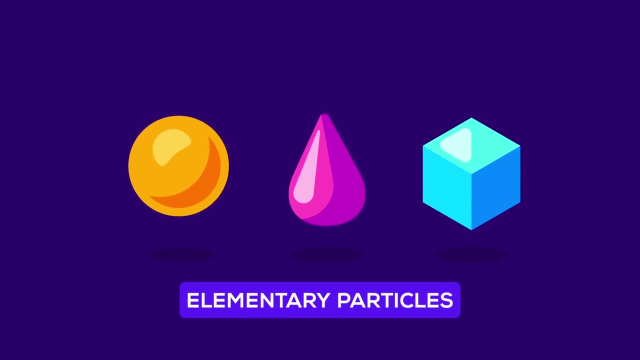 Atoms. We thought they were the final layer of reality until we smashed them together really hard and discovered things that can't be divided anymore: Elementary particles. But now we had a problem: They're so small that we could no longer look at them. 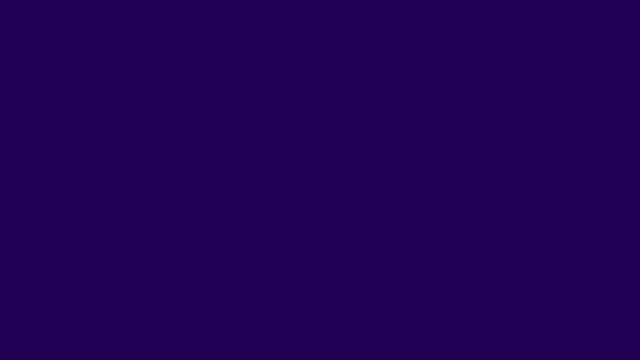 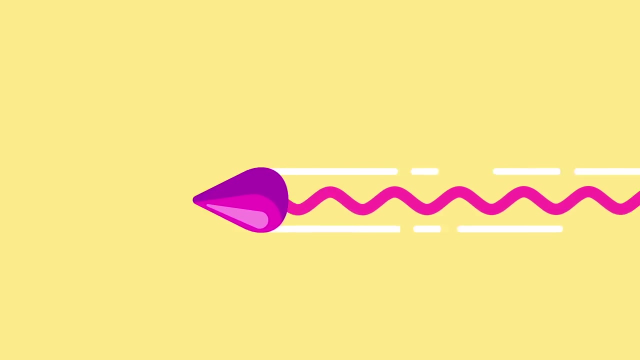 Think about it. What is seeing? To see something, we need light, an electromagnetic wave. This wave hits the surface of the thing and gets reflected back from it into your eye. The wave carries information from the object that your brain uses to create an image. 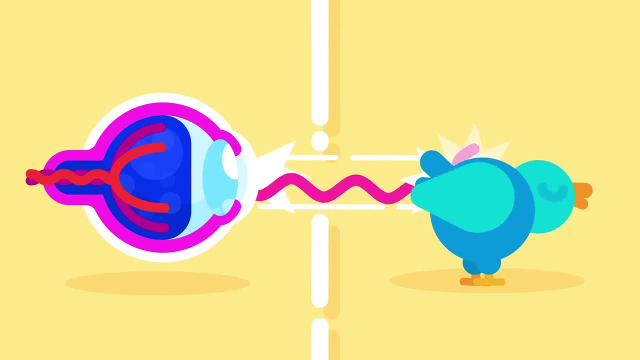 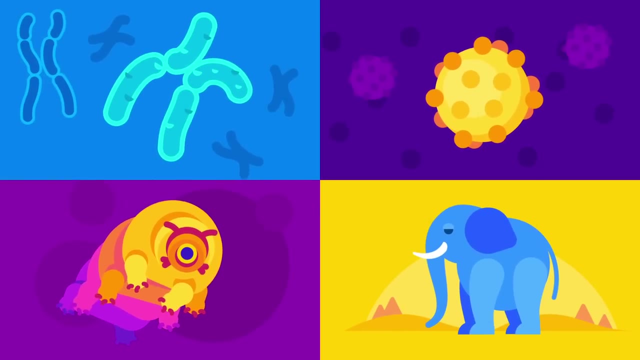 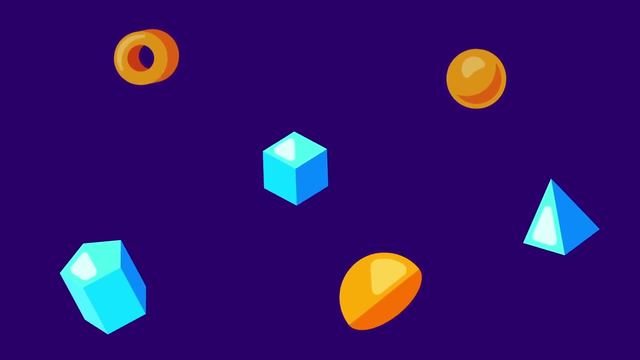 So you can't see something without somehow interacting with it. Seeing is touching An active process, not a passive one. This is not a problem with most things, But particles are very, very, very small- So small that the electromagnetic waves we use to see are too big to touch them. 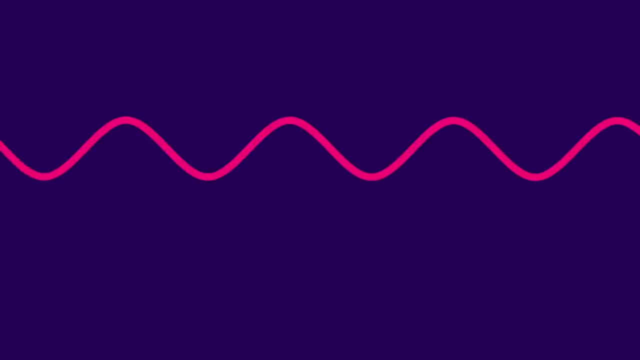 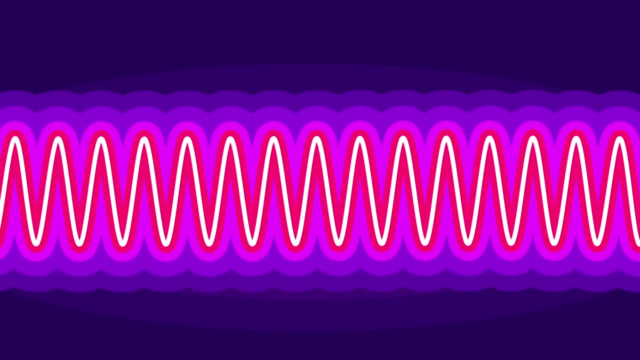 Visible light just passes over them. We can try to solve this by creating electromagnetic waves with more and much smaller wavelengths, But in quantum physics shorter wavelengths means more energy, So when we touch a particle with a wave that has a lot of energy, it gets a kick. 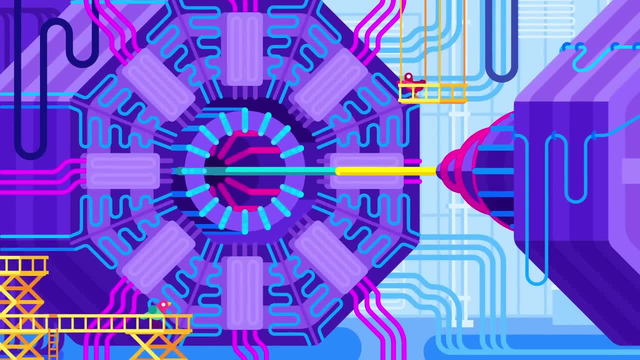 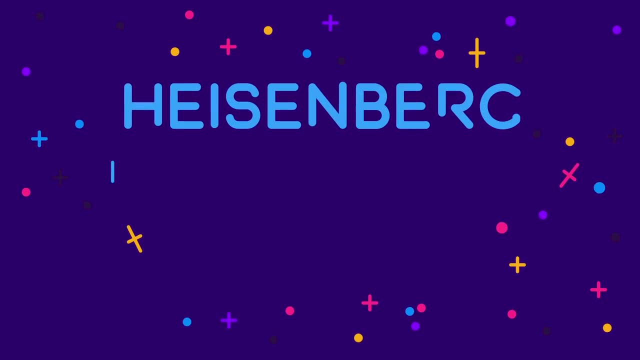 By looking at a particle, we change it. In quantum physics, we cannot know where a particle is and where it's going with absolute precision. This fact is so important that it has a name: The Heisenberg Uncertainty Principle, The basis of all quantum physics. 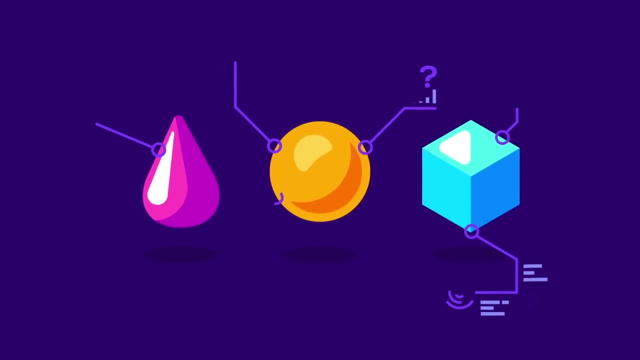 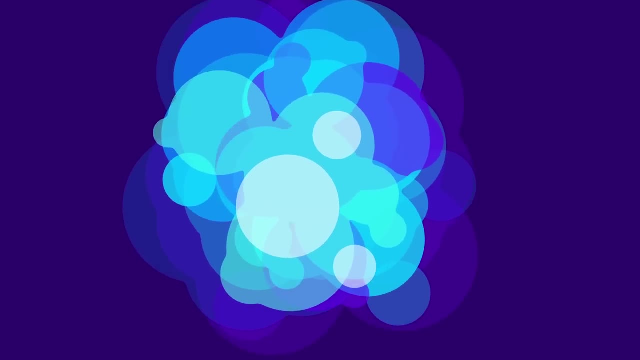 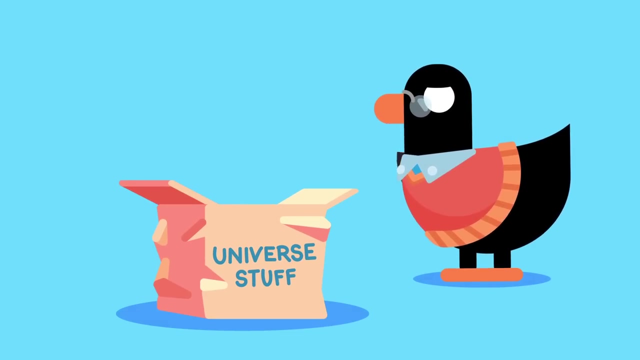 So what does a particle look like then? What is its nature? We don't know. If we look really hard, we can see a blurry sphere of influence, but not the particles themselves. We just know they exist. But if that's the case, how can we do any science with them? 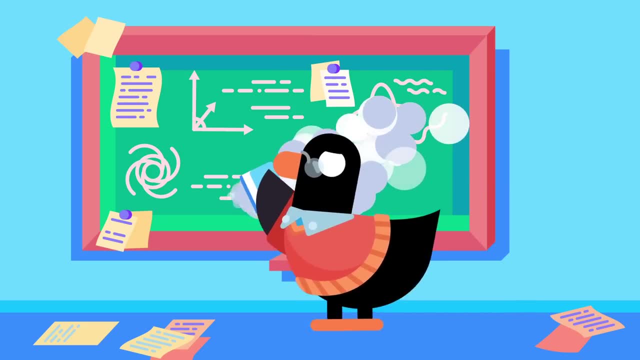 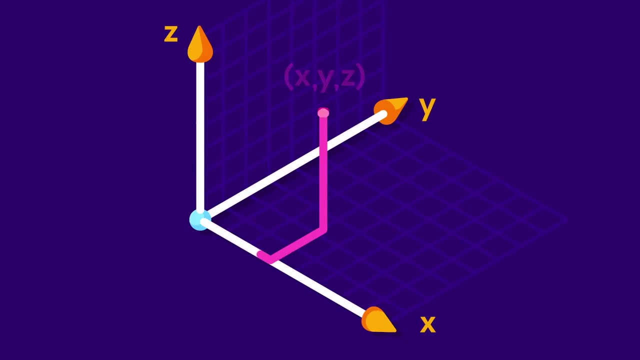 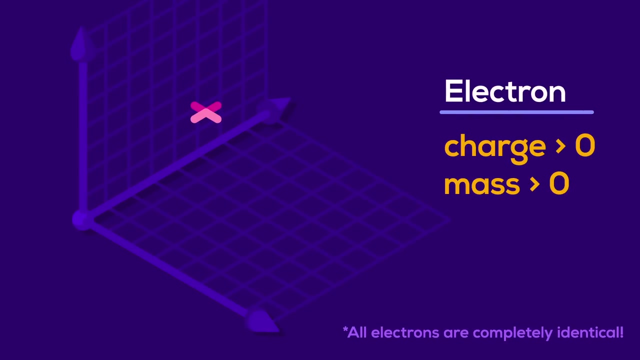 This is what humans do and invented a new story, a mathematical fiction, The story of the point particle. We decided that we would pretend that a particle is a point in space. Any electron is a point with a certain electric charge and a certain mass, all indistinguishable from each other. This way, physicists could define them and calculate all of their interactions. This can be made precise in quantum field theory and this solved a lot of problems. All of the standard model of particle physics is built on it and it predicts lots of things very well. 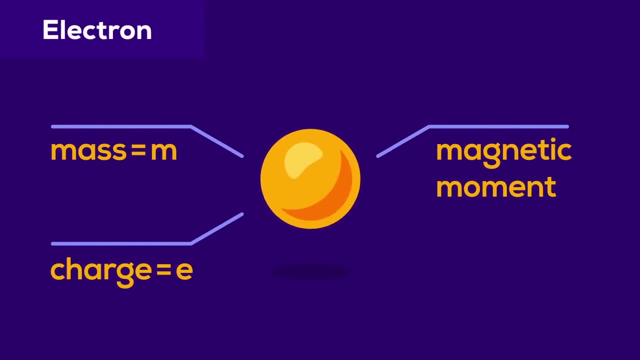 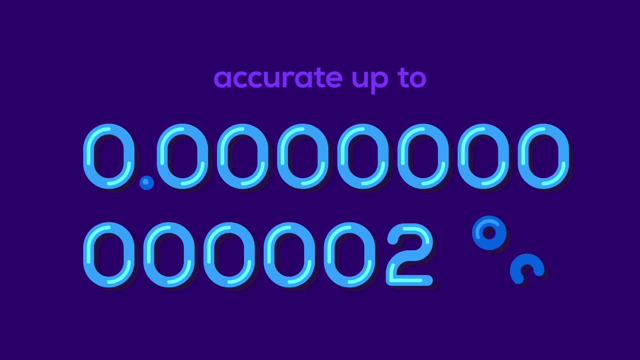 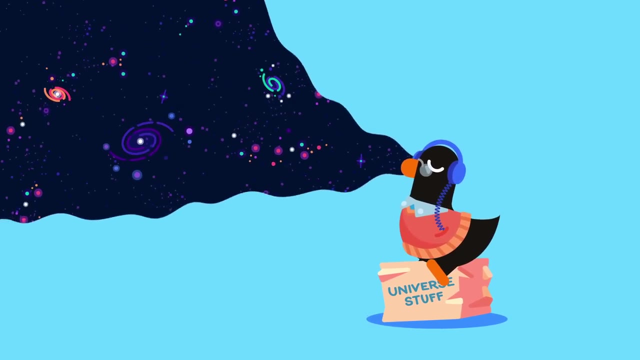 Some quantum properties of the electron, for example, have been tested and are accurate up to 0.000000000000002%. So, while particles are not really points, by treating them as if they were, we get a pretty good picture of the universe. 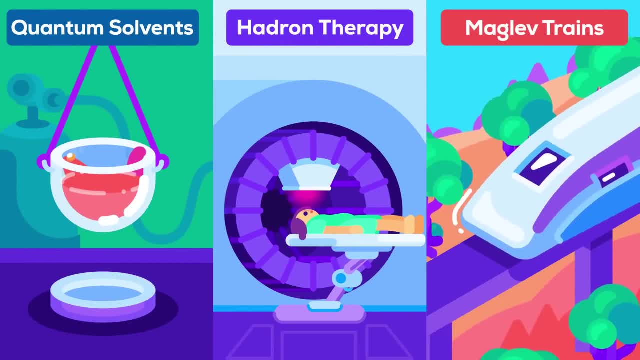 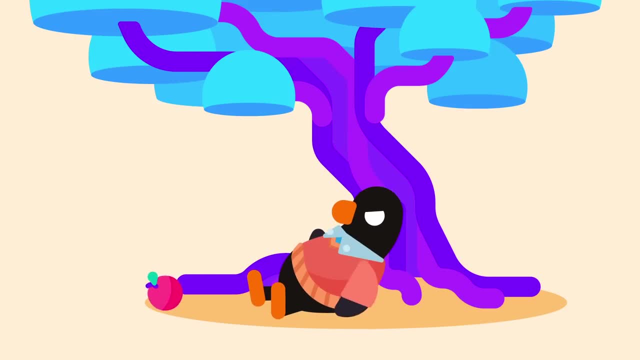 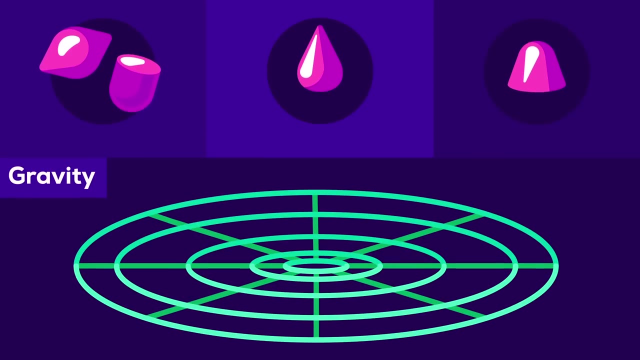 Not only did this idea advance science, it also led to a lot of real-world technology we use every day. But there's a huge problem: gravity. In quantum mechanics, all physical forces are carried by certain particles, But according to Einstein's general relativity, gravity is not a force like the others in the universe. 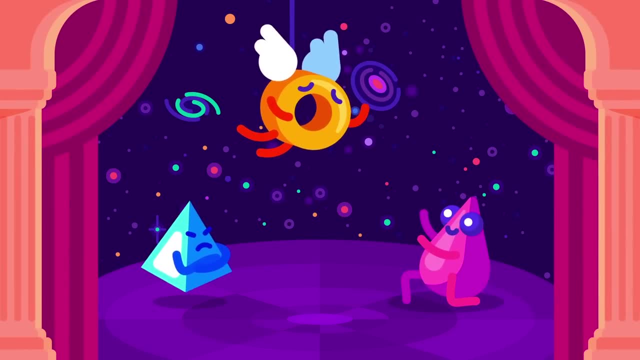 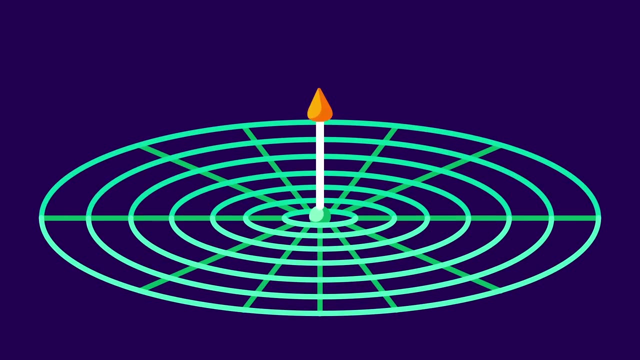 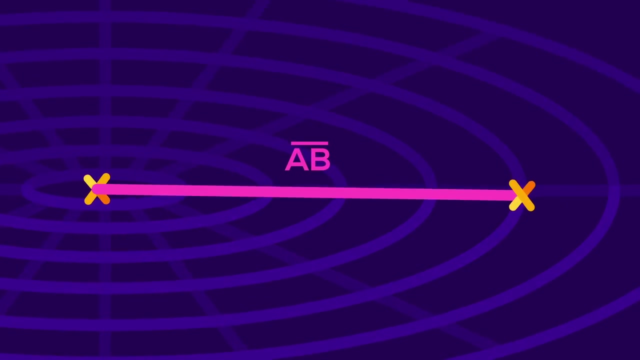 If the universe is a play, particles are the actors, but gravity is the stage. To put it simply, gravity is a theory of geometry, the geometry of space-time itself, of distances, which we need to describe with absolute precision. But since there is no way to precisely measure things in the quantum world, 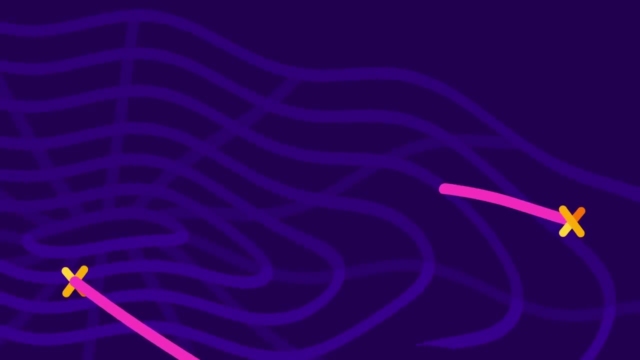 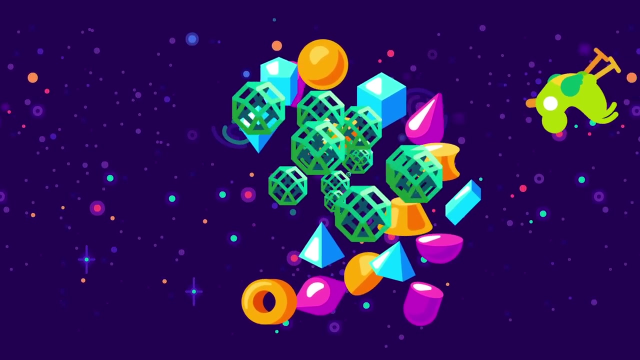 our story of gravity doesn't work with our story of quantum physics. When physicists tried to add gravity to the story by inventing a new particle, their mathematics broke down, And this is a big problem. If we could marry gravity to quantum physics and the standard model, 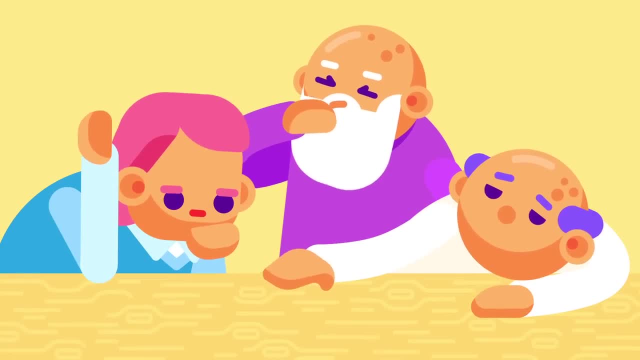 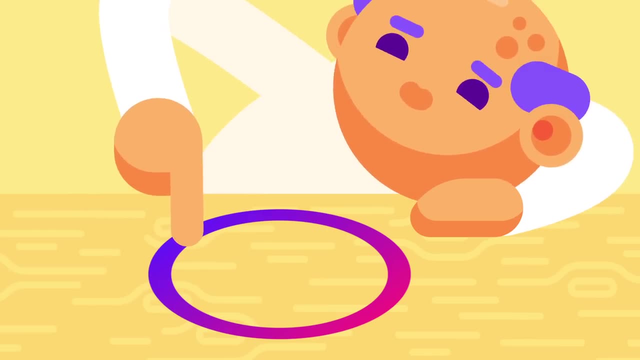 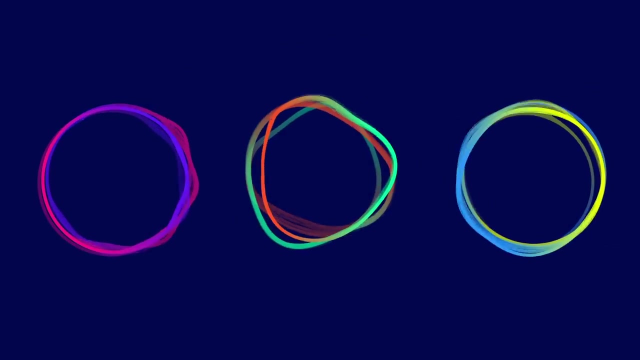 we would have the theory of everything. So very smart people came up with a new story. They asked: what is more complex than a point, a line or a string? String theory was born. What makes string theory so elegant is that it describes many different elementary particles. 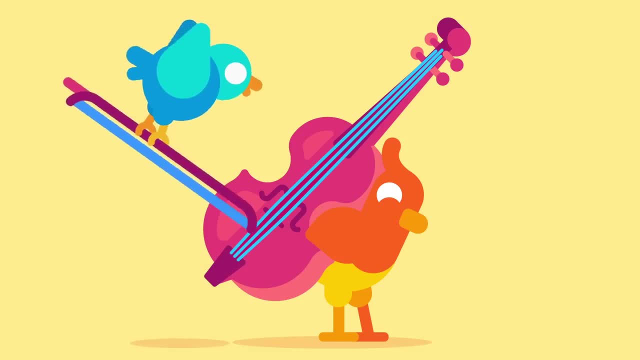 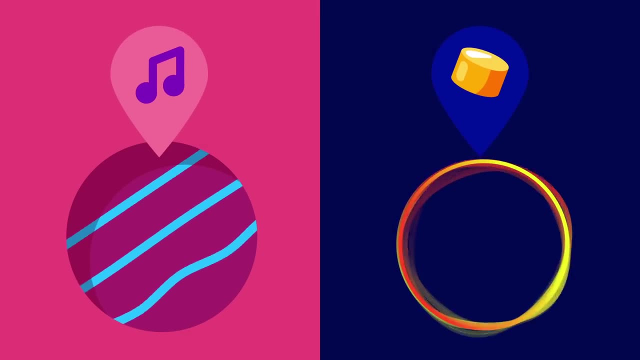 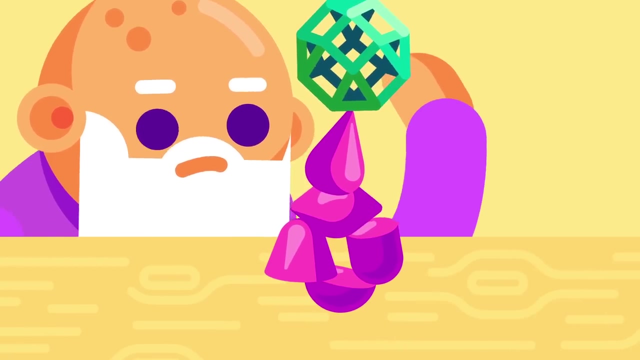 as different modes of vibration of the string. Just like a violin string vibrating differently can give you a lot of different notes, a string can give you different particles. Most importantly, this includes gravity String theory. promised to unify all fundamental forces of the universe. 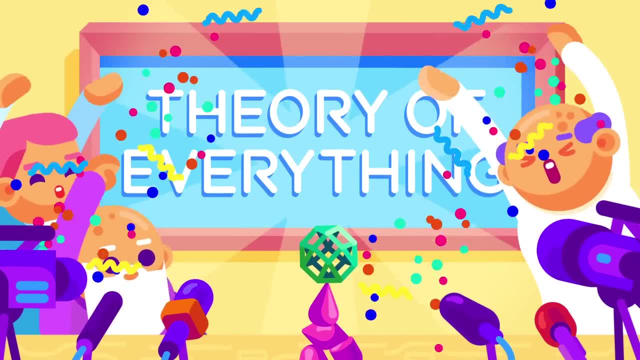 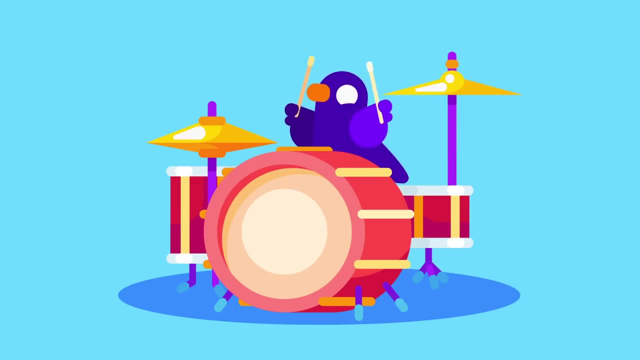 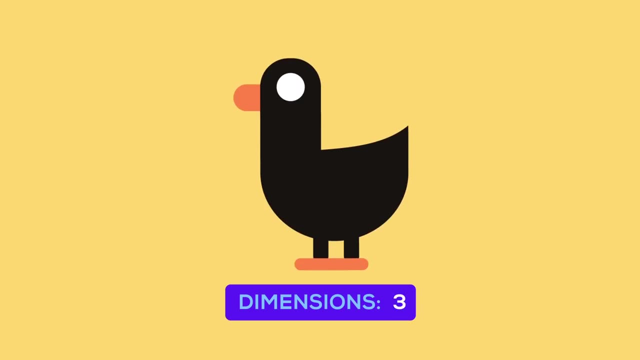 This caused enormous excitement and hype. String theory quickly graduated to a possible theory of everything. Unfortunately, string theory comes with a lot of strings attached. Much of the maths involving a consistent string theory does not work in our universe with its three spatial and one temporal dimensions. 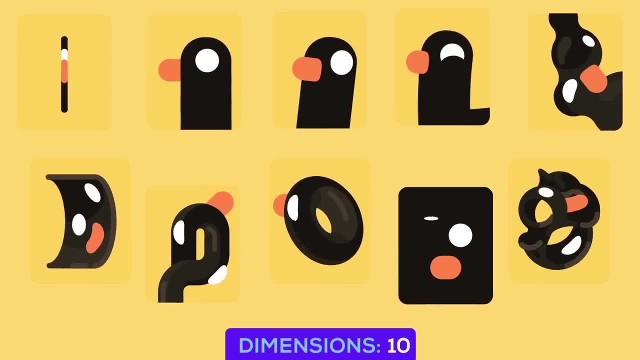 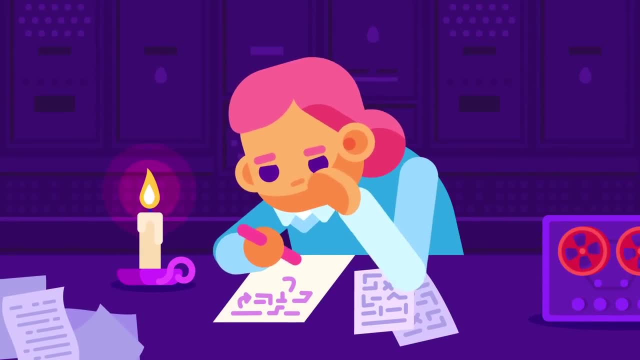 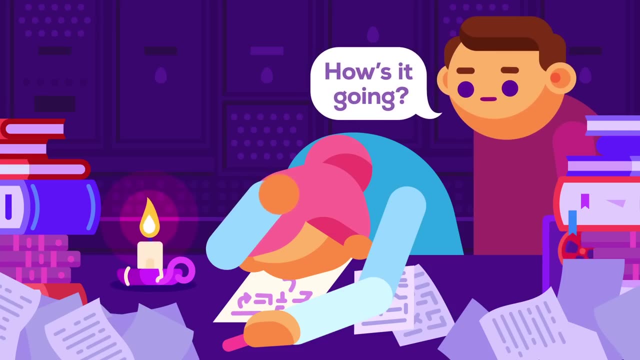 String theory requires ten dimensions to work out. So string theorists do calculations in model universes and then try to get rid of the six additional dimensions and describe our own universe. But so far nobody has succeeded and no prediction of string theory has been proven in an experiment. 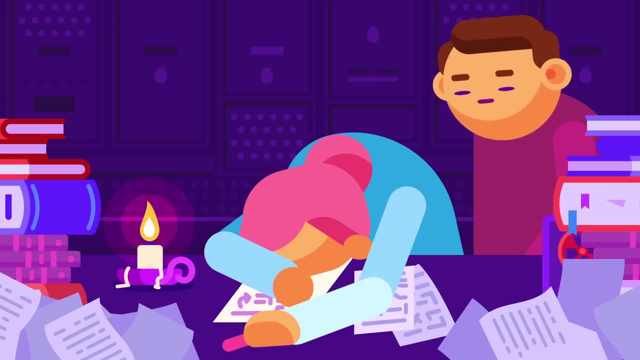 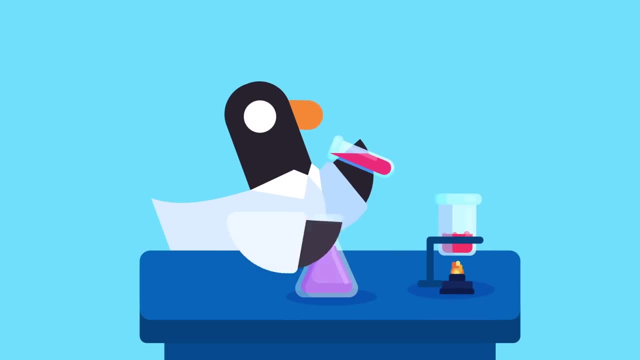 So string theory did not reveal the nature of our universe. One could argue that in this case, string theory really isn't useful at all. Science is all about experiments and predictions. If we can't do those, why should we bother with strings? 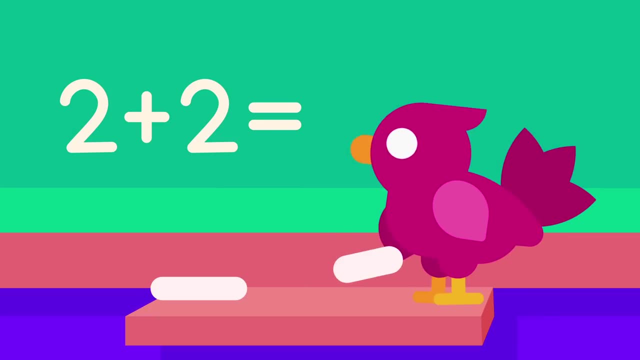 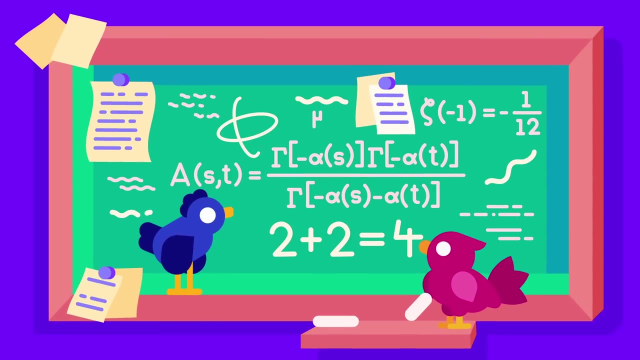 It really is all about how we use it. Physics is based on maths. Two plus two makes four. This is true no matter how you feel about it, And the maths in string theory does work out. That's why string theory is still useful. 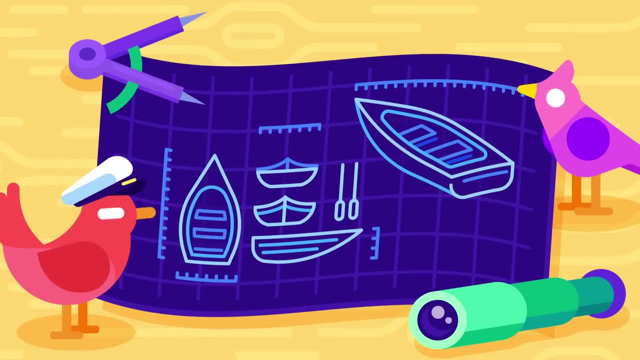 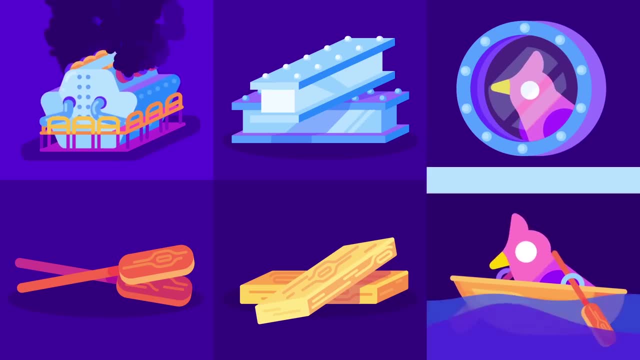 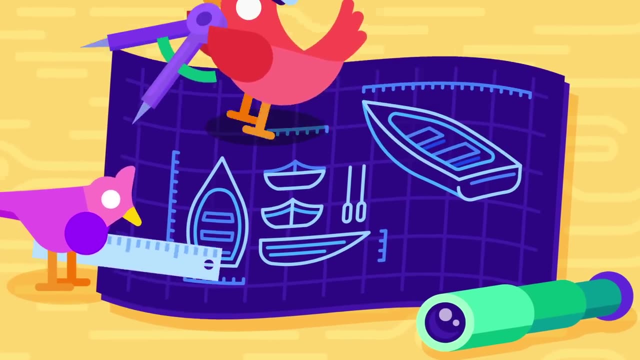 Imagine that you want to build a cruise ship but you only have blueprints for a small rowing boat. There are plenty of differences- The engine, the materials, the scale- But both things are fundamentally the same- Things that float. So by studying the rowing boat blueprints, 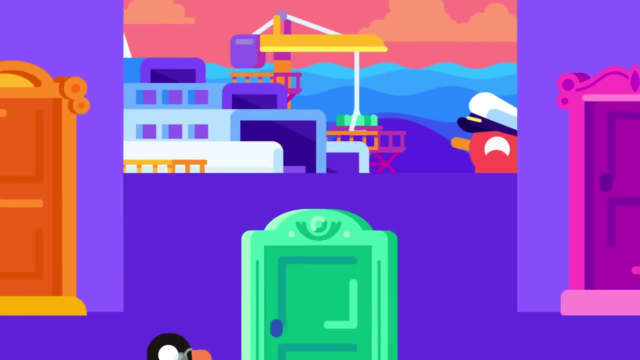 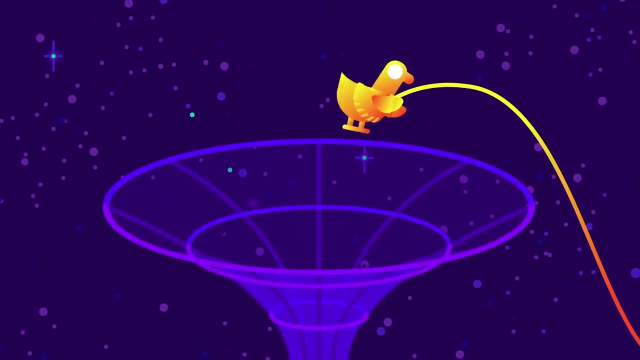 you might still learn something about how to build a cruise ship. eventually, With string theory, we can try to answer some questions about quantum gravity that have been puzzling physicists for decades, such as how black holes work or the information paradox. String theory may point us in the right direction. 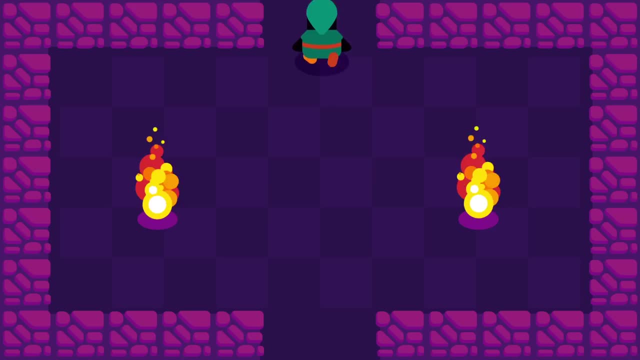 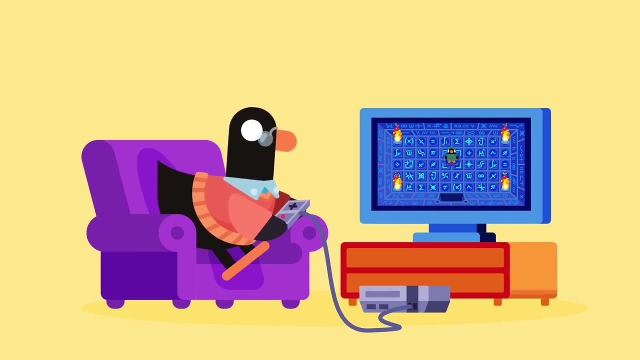 When used in this spirit, string theory becomes a precious tool for theoretical physicists and help them discover new aspects of the quantum world and some beautiful mathematics. So maybe the story of string theory is not the theory of everything, But just like the story of the point particle. 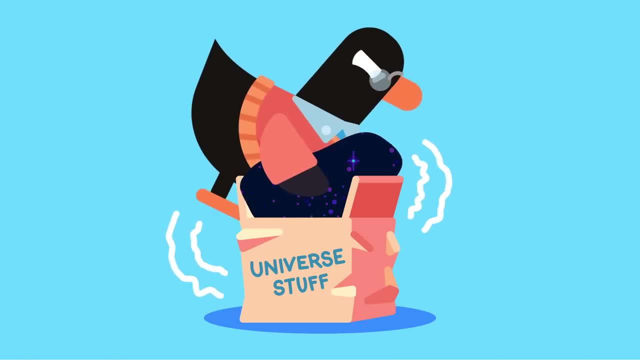 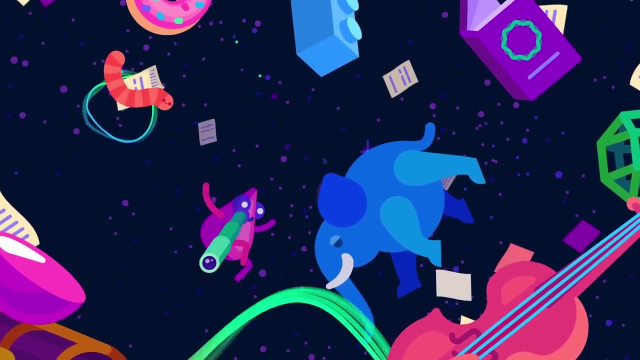 it may be an extremely useful story. We don't yet know what the true nature of reality is, but we'll keep coming up with stories to try and find out until one day. hopefully, we do know. This video was supported by the Swiss National Science Foundation.